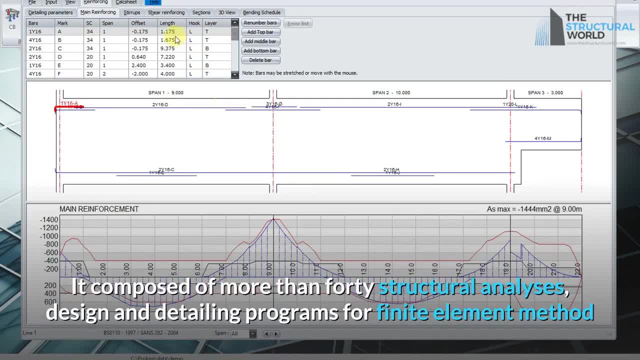 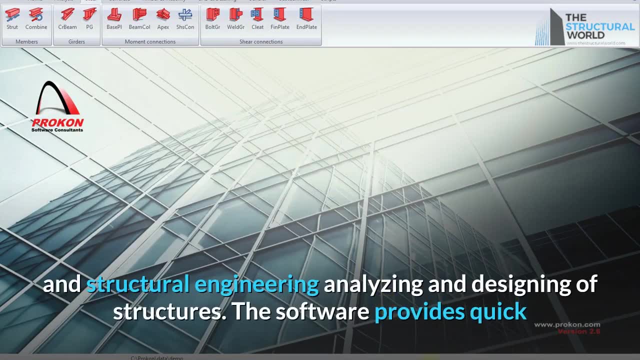 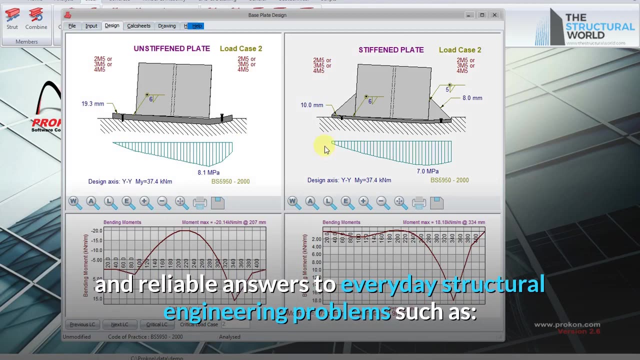 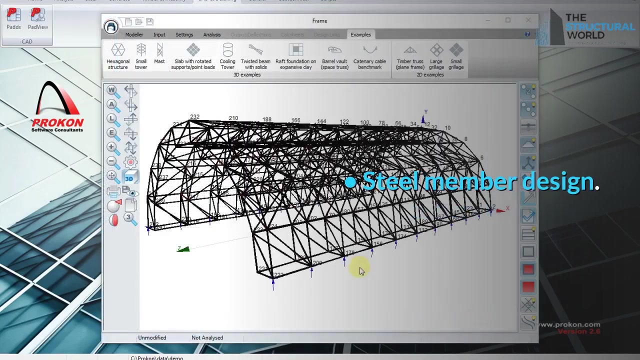 it is widely used worldwide. It composed of more than 40 structural analyses, design and detailing programs for finite element method and structural engineering analyzing and designing of structures. The software provides quick and reliable answers to everyday structural engineering problems, such as Reinforced and pre-stressed concrete design, Steel member design, Steel connection design, Frame and finite 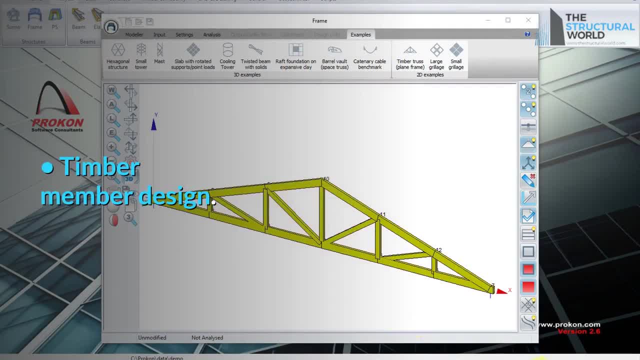 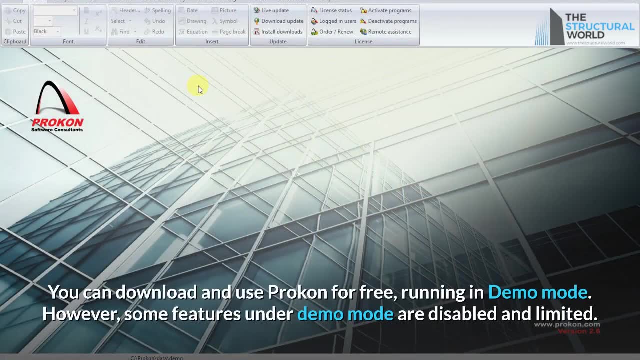 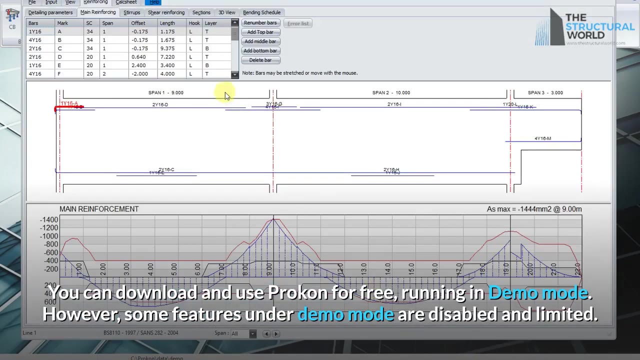 element analysis: Timber member design, Masonry design, CAD and reinforced concrete detailing. You can download and use Procon for free running in demo mode. However, some features under demo mode are disabled and limited, But you can still use the demo mode in no time. However, some features under demo mode are disabled and limited, But you can still use the demo mode in no time. 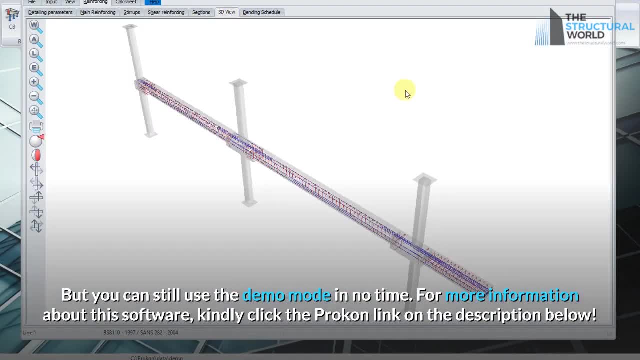 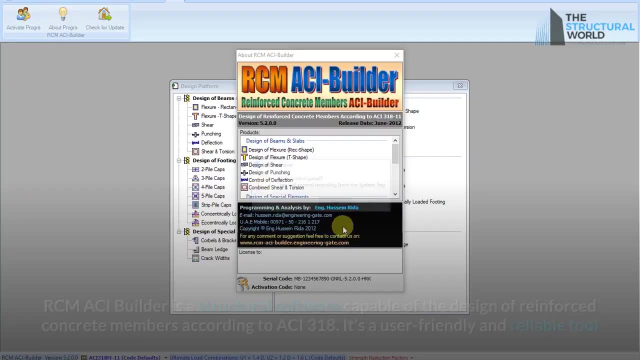 However, some features under demo mode are disabled and limited, But you can still use the demo mode in no time. For more information about this software, kindly click the Procon link on the description below 2. RCMACI Builder. RCMACI Builder is a structural software. 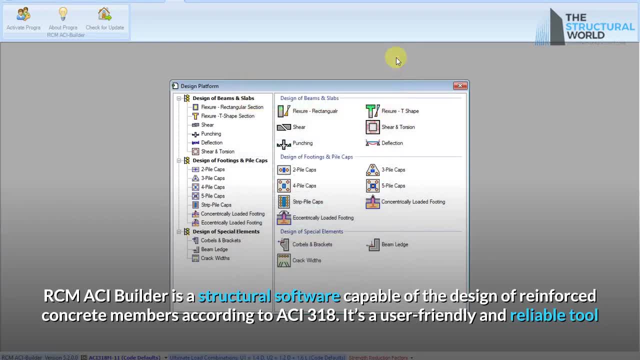 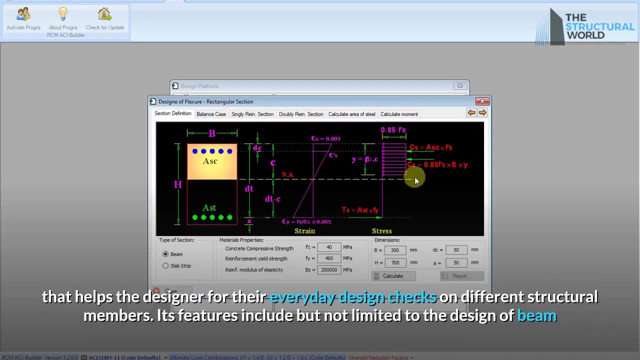 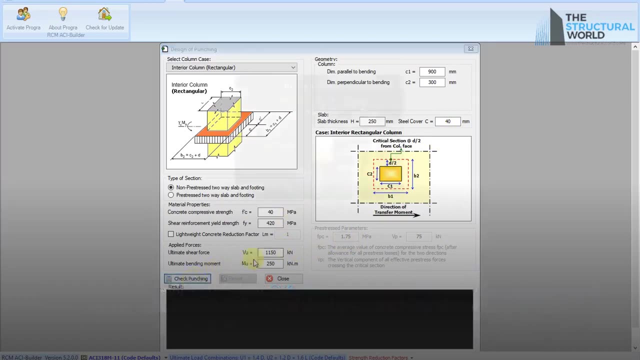 capable of the design of reinforced concrete members according to ACI 318.. It's a user-friendly and reliable tool that helps the designer for their everyday design checks on different structural members. Its features include, but not limited to, the design of beam and slabs, which includes flexural design, punching, shear and deflection. 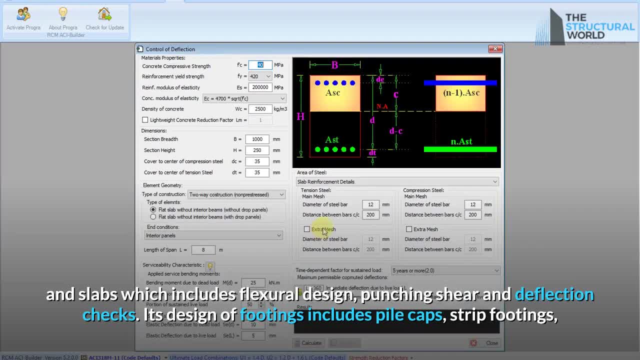 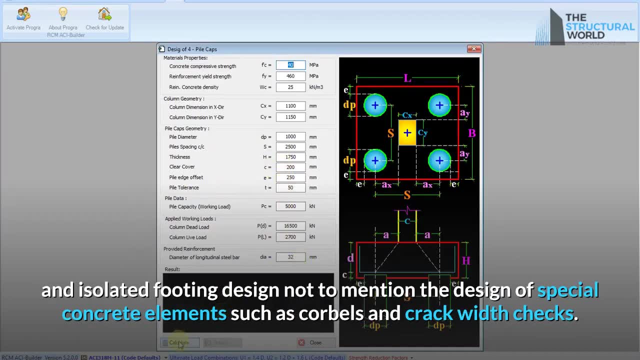 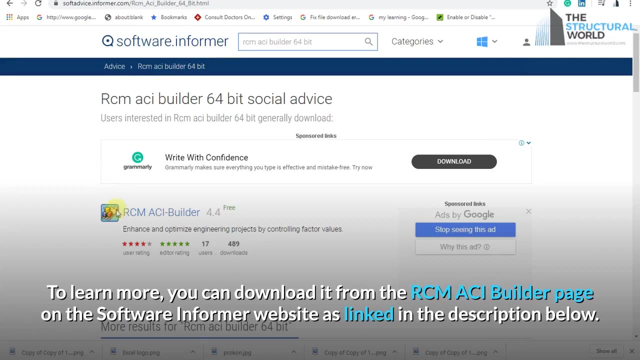 checks. Its design of footings includes pile caps, strip footings and isolated footing design, not to mention the design of special concrete elements such as corbels and crack width checks. To learn more, you can download it from the RCMACI Builder page on the Software. 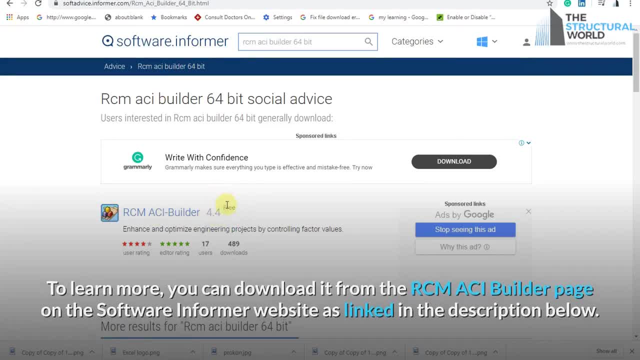 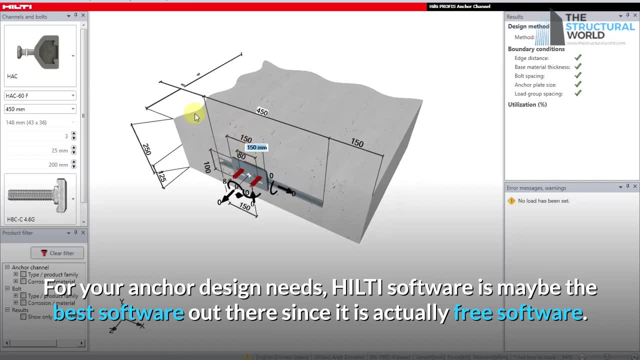 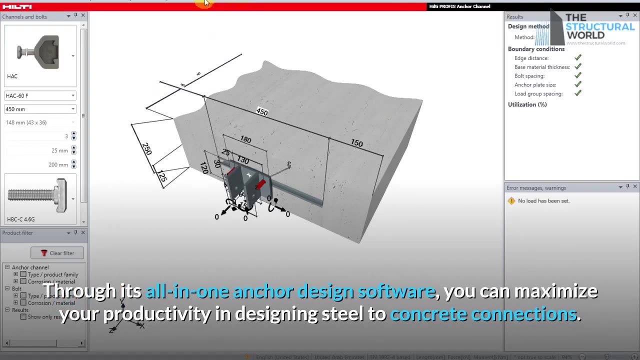 Informer website, as linked in the description below 3. Hilti Software For your anchor design needs. Hilti software is maybe the best software out there, since it is actually free software. Through its all-in-one anchor design software, you can maximize your. 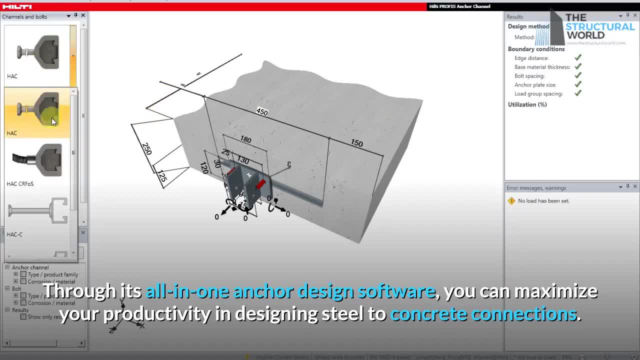 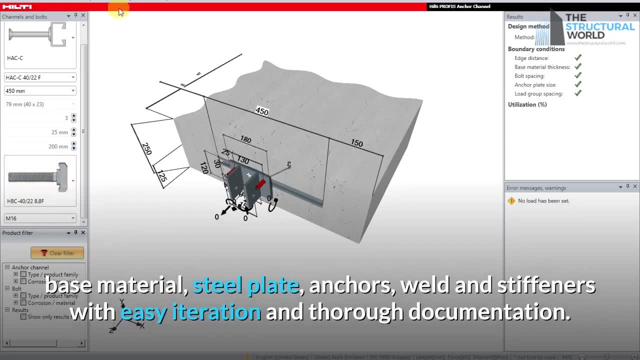 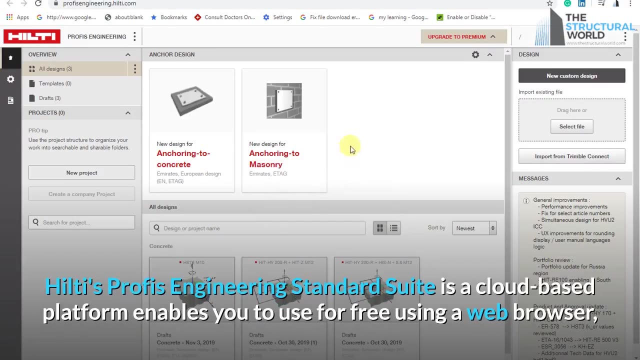 productivity in designing steel-to-concrete connections. It handles calculations and analysis of the different elements of a steel-to-concrete connection, including base material, steel plate, anchors, weld and stiffeners, with easy iteration and thorough documentation. Hilti's PROFIS Engineering Standard Suite is a cloud-based platform enables you to use for free. 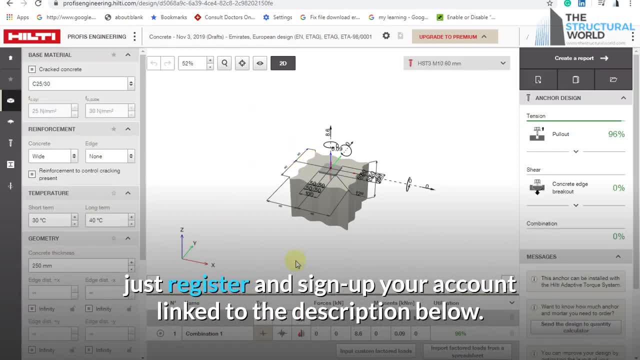 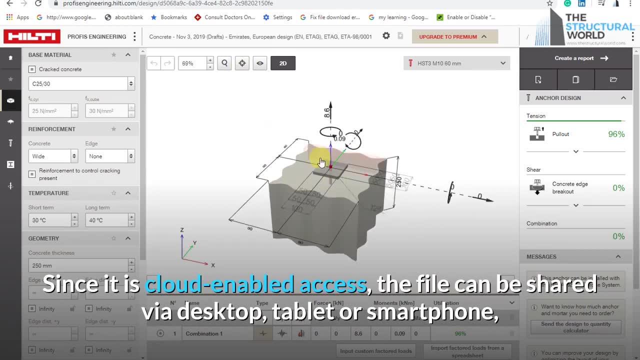 using a web browser: just register and sign up your account linked to the description below. Since it is cloud-enabled access, the file can be shared via desktop, tablet or smartphone. it can only use by logging in into your account, not unless you upgrade it into a premium version. 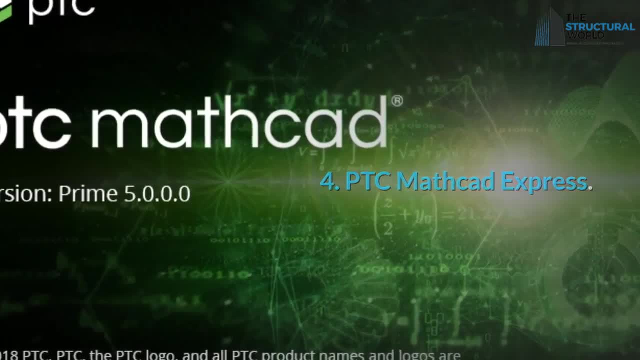 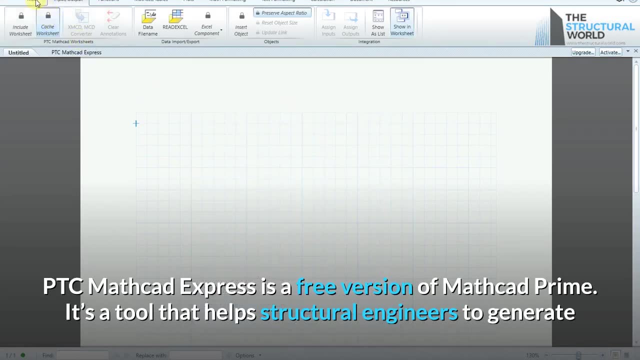 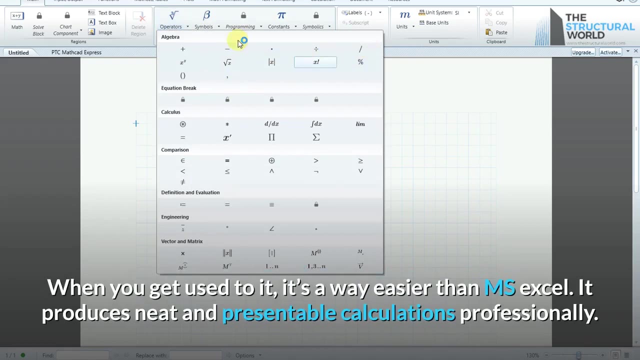 4. PTC Mathcad Express. PTC Mathcad Express is a free version of Mathcad Prime. It's a tool that helps structural engineers to generate and produce professional-quality hand calculations, from simple to complex, When you get used to it. 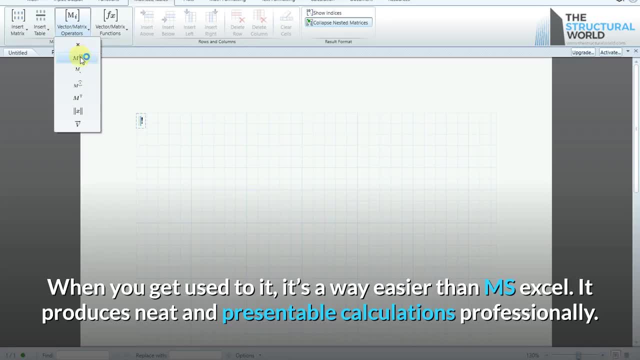 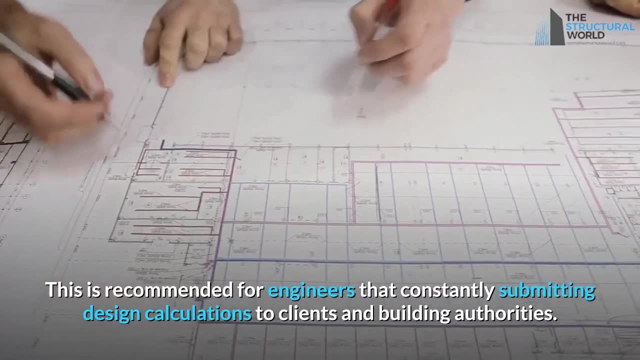 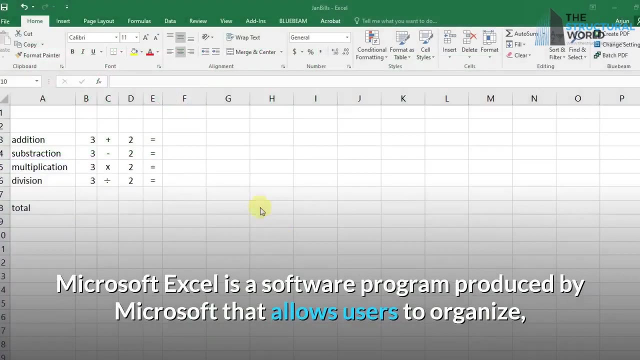 it's a way easier than MS Excel. It produces neat and presentable calculations professionally. This is recommended for engineers that constantly submitting design calculations to clients and building authorities. 5. MS Excel- Microsoft Excel. Excel is a software program produced by Microsoft that allows users to organize. 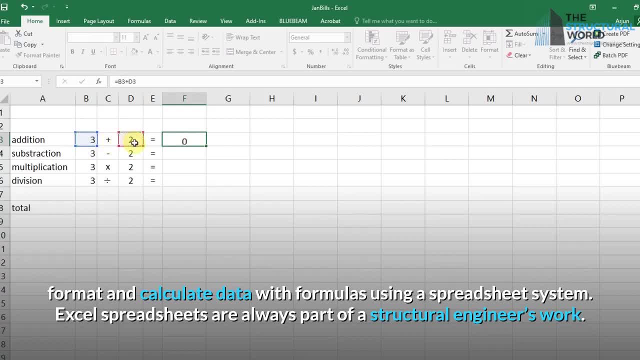 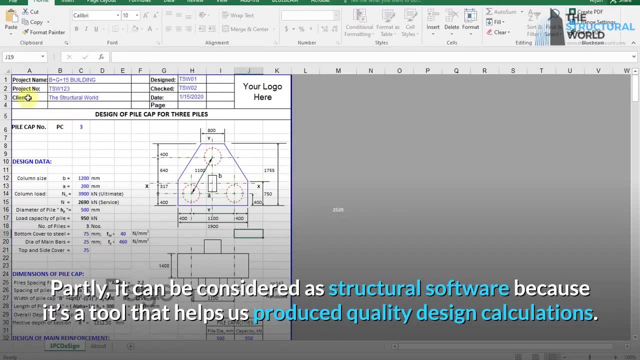 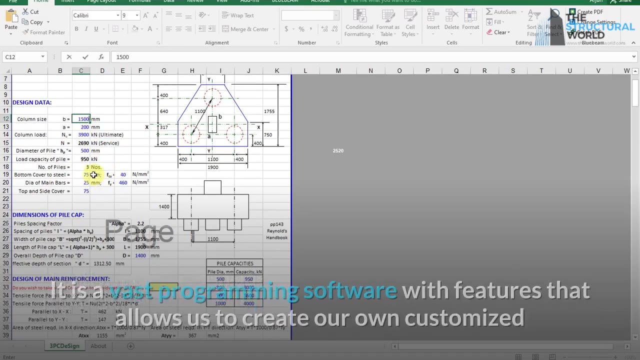 format and calculate data with formulas using a spreadsheet system. Excel spreadsheets are always part of a structural engineer's work. Partly it can be considered as structural software because it's a tool that helps us produce quality design calculations. It is a vast programming software with features that 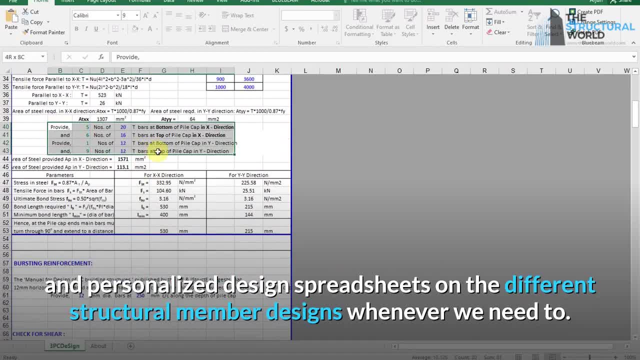 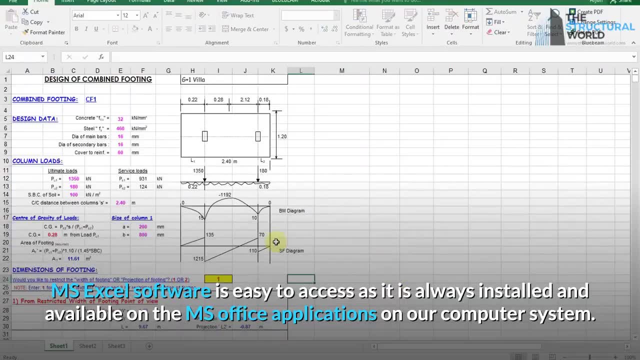 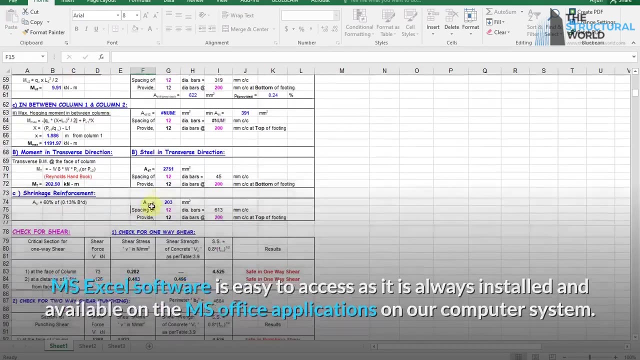 allows us to create our own customized and personalized design spreadsheets on the different structural member designs whenever we need to. MS Excel software is easy to access as it is always installed and available on the MS Office applications on our computer system. Any of the free structural software that we haven't discussed that you know of. 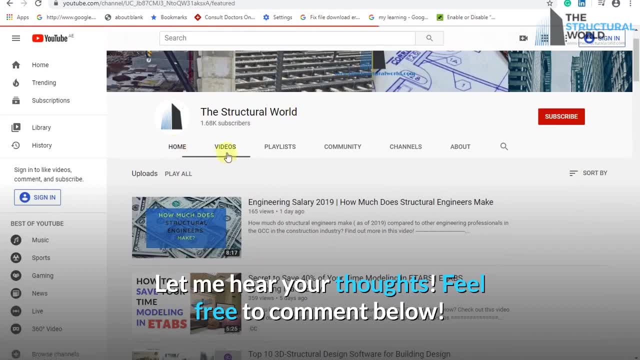 Let me hear your thoughts. Feel free to comment below. Thanks for watching. Don't forget to like, share and subscribe. Thanks for watching. Don't forget to like, share and subscribe.